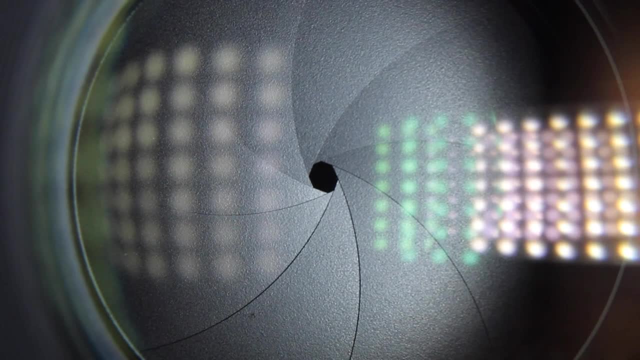 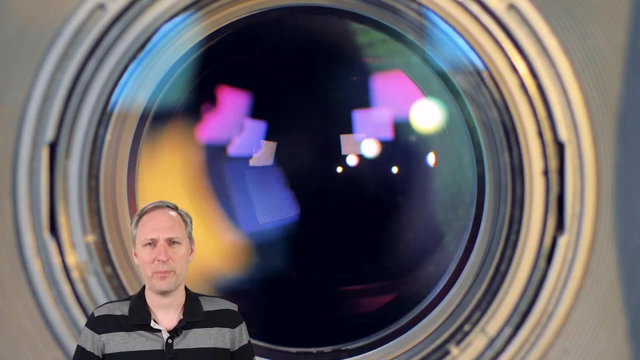 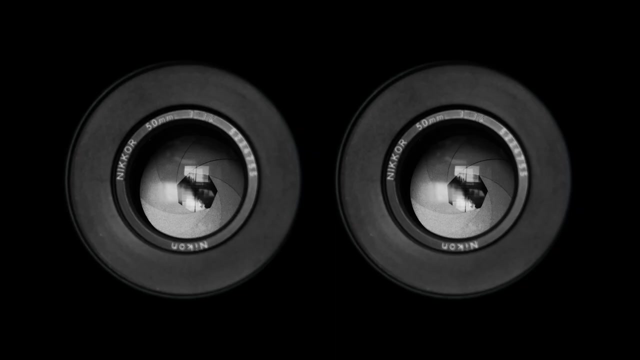 started. Cameras are a very popular option for robots because of their similarity to human eyes, their relatively low cost and the abundance of algorithms for extracting information. Robots need to be able to sense their surroundings and a common way of them detecting information from pictures. One such algorithm is the stereo vision algorithm. This 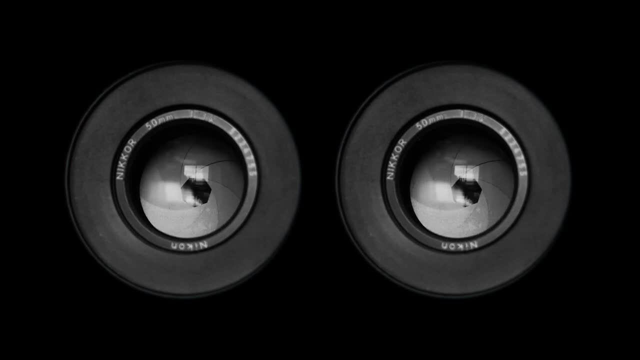 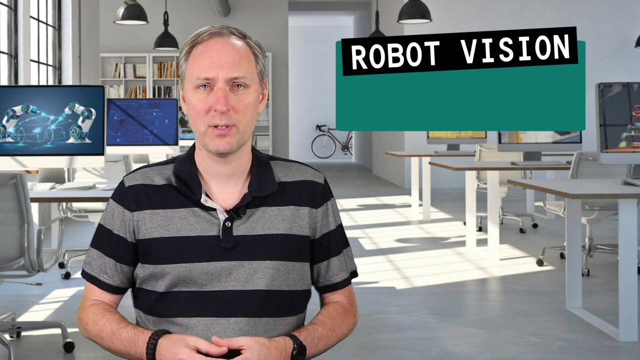 algorithm allows the robot, using two cameras, to calculate the distance to nearby objects. For example, our robot can use stereo imagery to avoid running into a tree as it drives around. To explore this aspect of robot vision, we will follow three steps. Step one: take a picture. 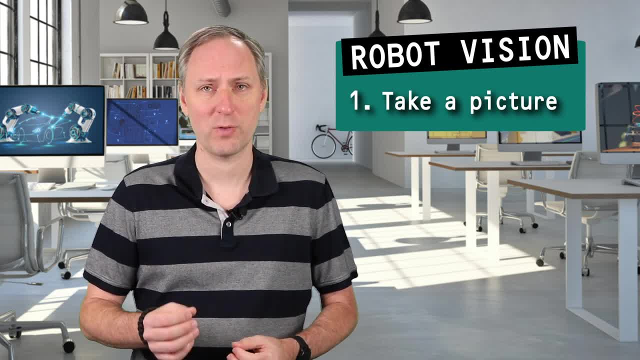 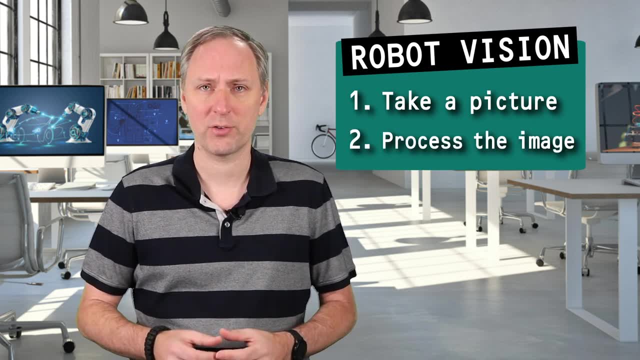 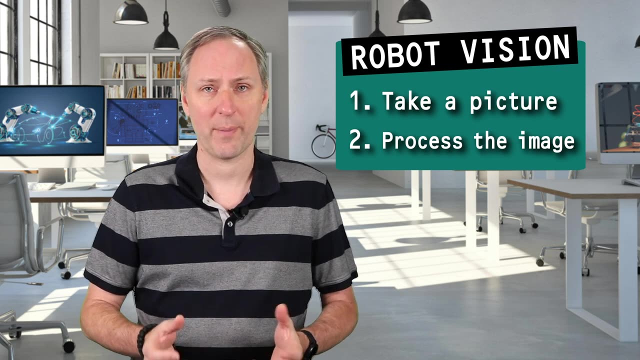 This step produces an image, a two-dimensional image and a two-dimensional representation of the real world. Step two: process the image. Find interesting points such as corners and edges of objects in the image. We'll call these interesting points features. Step three: calculate information. Use the features to extract information about the 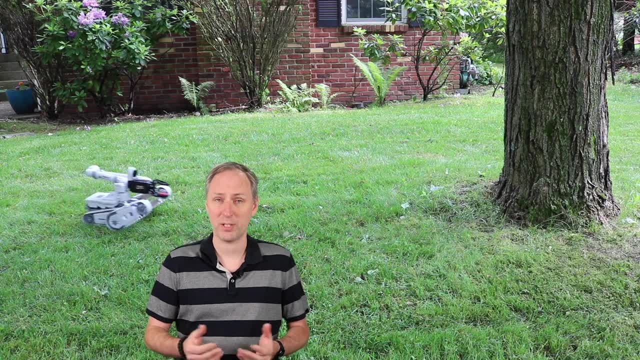 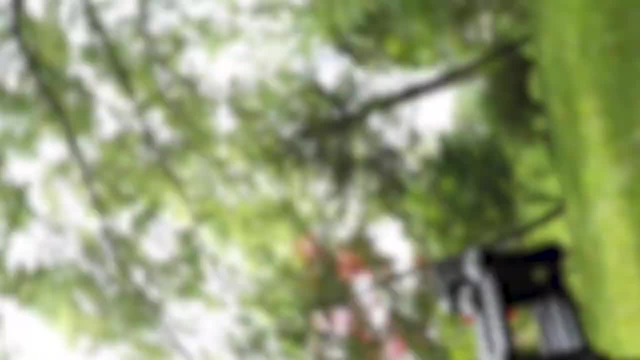 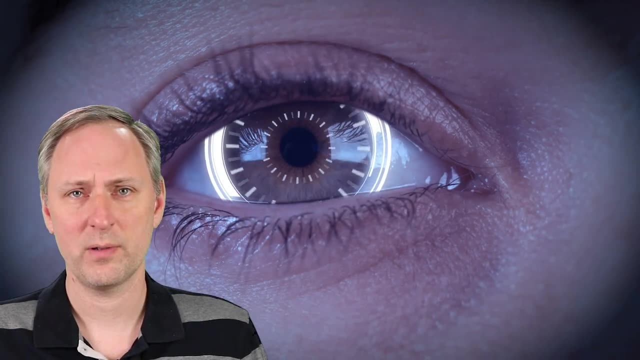 scene, such as where objects are or the distance to particular features or which objects are in view. Step four: be sure to mention that theAND has functioned within the first three sets. Hey robot, See that tree To better understand robot vision. then compare robot cameras. 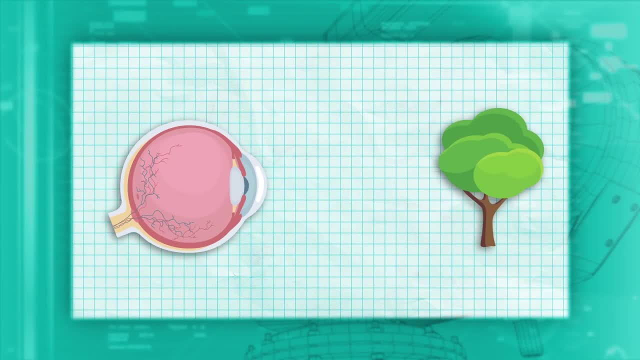 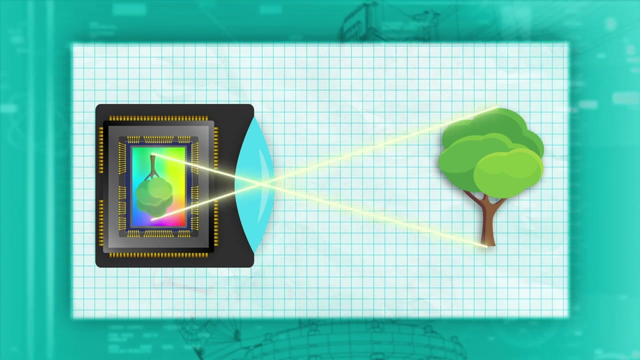 to your eyes In order to see an object in front of you. light from a light source bounces off the object and goes through the lens in your eye and forms an image on your retina. The robot's camera eye works the same way: Light bounces off an object, goes through the camera's. 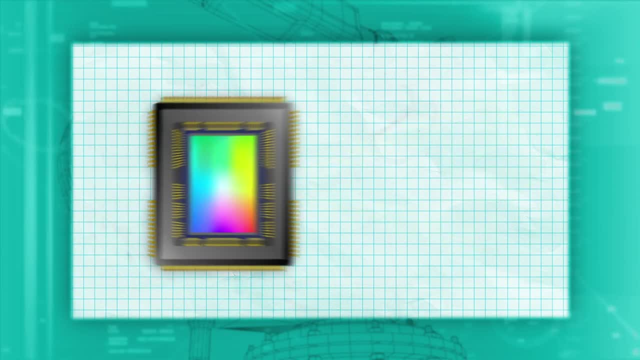 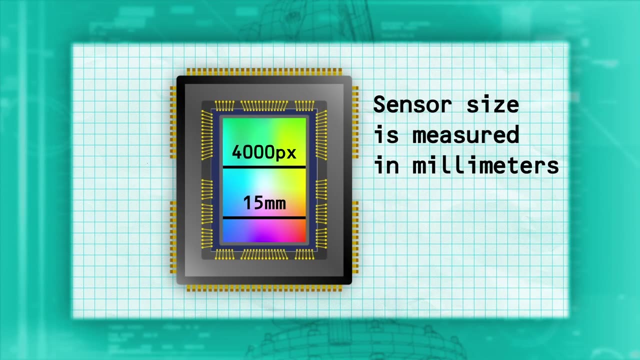 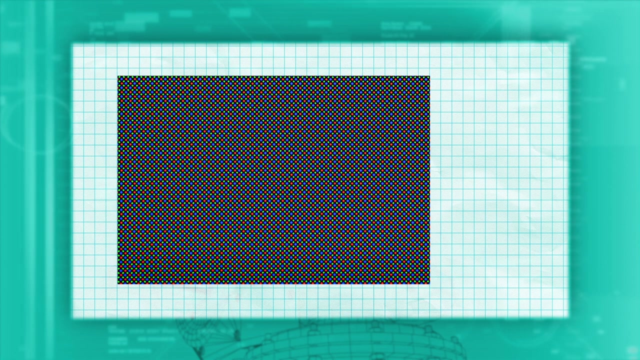 lens and forms an image on the sensor. The camera sensor itself is fairly small. Usually these sensors are measured in millimeters and are about the size of a fingernail, but can be slightly bigger or much smaller. The sensor is made up of a grid of very small individual color sensors, similar to the cone. 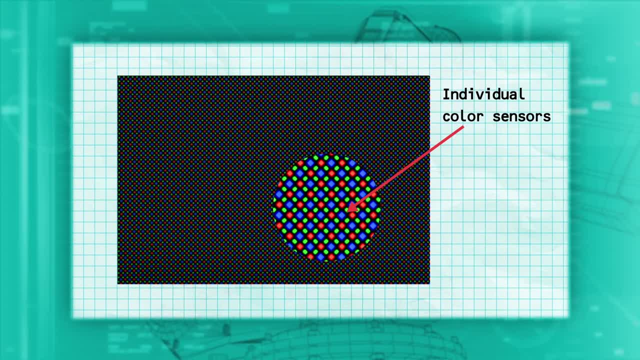 cells in your eyes. These small sensors are known as pixels, a term you've probably heard before. Each pixel measures the color of one tiny point in the image. When you put all the small points of color together, you get the full image. 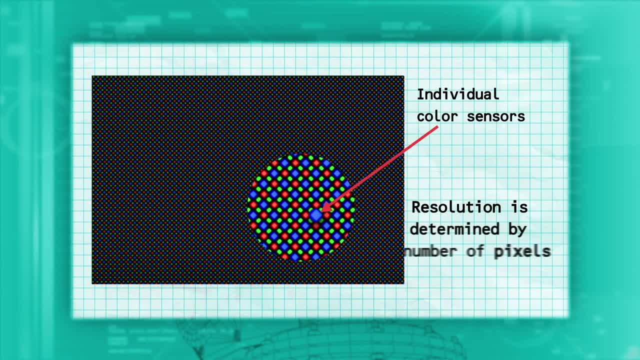 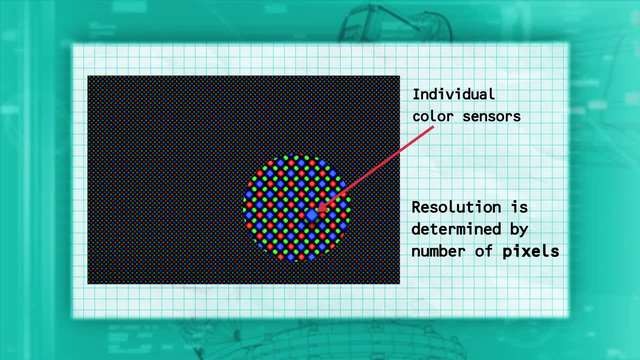 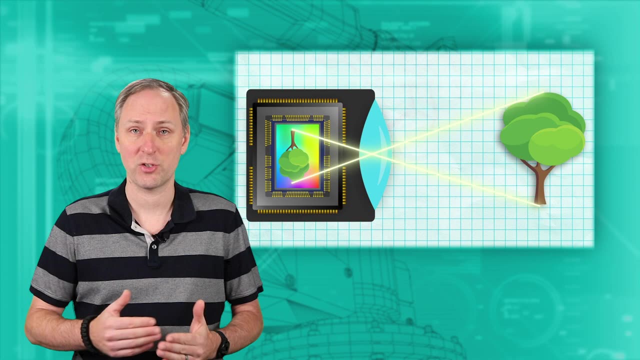 The number of these small sensors or pixels determines the resolution of the camera, And for a typical camera there can be millions of pixels. Besides the resolution and sensor size, the other critical dimension of a camera is how far the image sensor is from the lens of the camera. 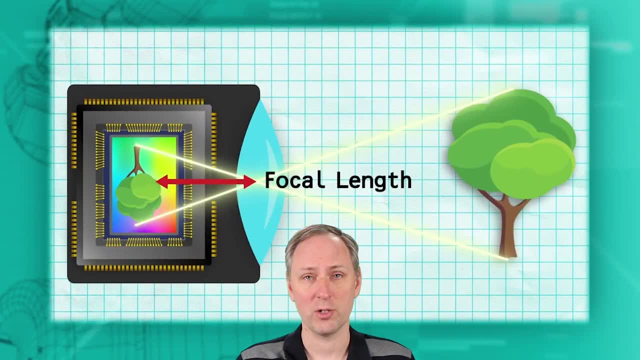 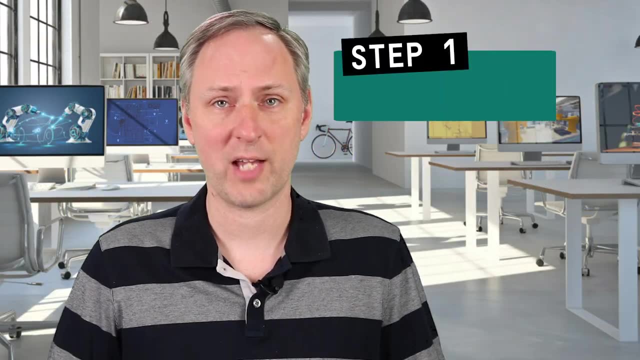 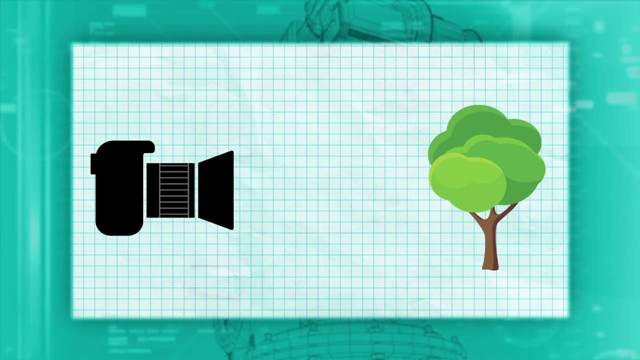 This distance is called the focal length of the camera. We can use the focal length information later to help us determine an object's location. Now let's look at an example to see how we accomplish our first step: taking a picture. We have our camera and an object, in this case a tree. 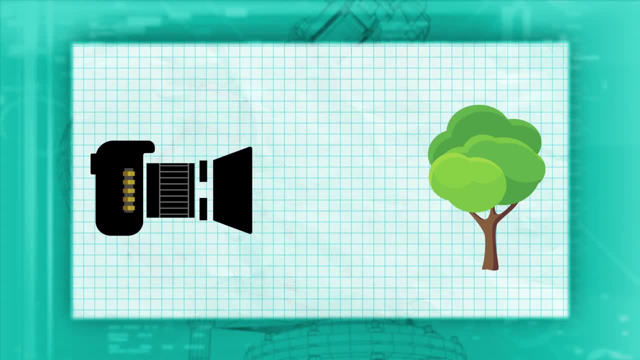 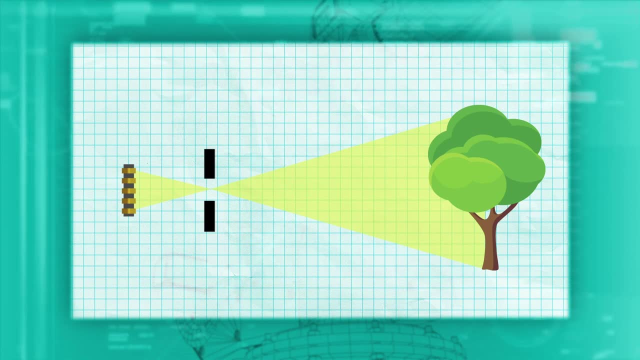 If we look inside the camera, we can see the sensor and the lens. Imagine the lens as a simple pinhole. We can see that the image is formed on the sensor. We can also think of the pinhole as the camera center. This model of camera is called the pinhole model. 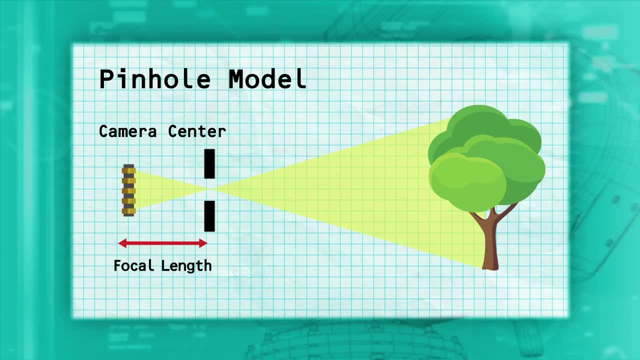 We can also see why the tree is upside down on the sensor, since the pinhole takes a ray from the top part of the tree and focuses it on the lower part of the sensor, and vice versa. Dealing with an upside down image isn't very convenient. 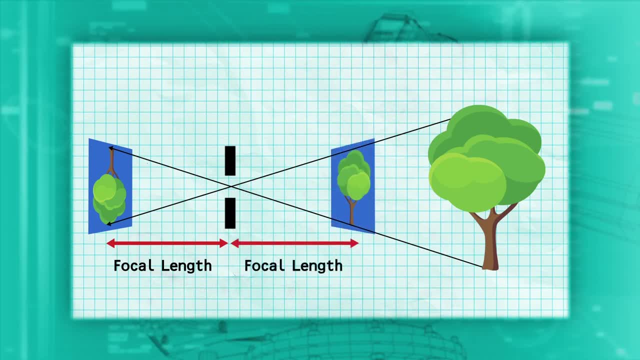 So what if we were to imagine an image in front of the pinhole, at the distance equal to the focal length, instead of behind the hole? Since the rays from the tree would now pass through the image plane before they went through the pinhole, we would get a right side up image. 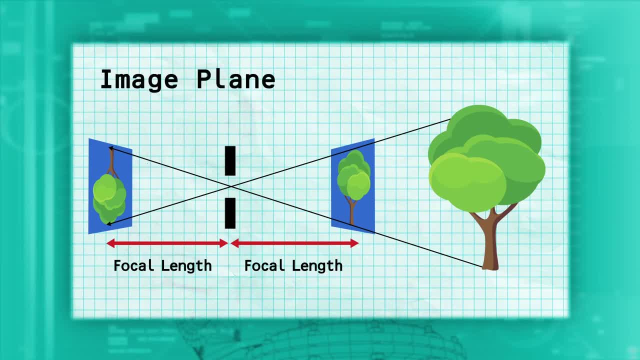 We call this new image the image plane, and it's almost always used instead of the actual image on the sensor when describing what the robot sees. Now that we have our image of the tree, we need to figure out what to do with it. 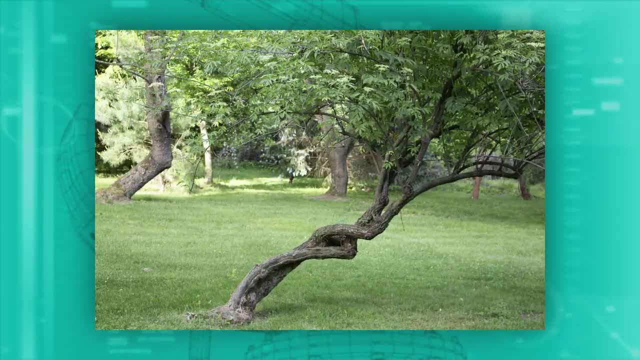 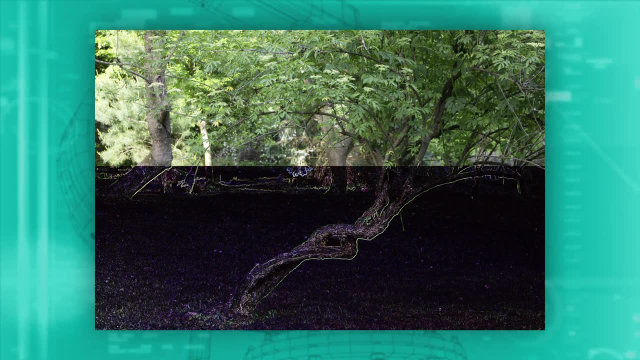 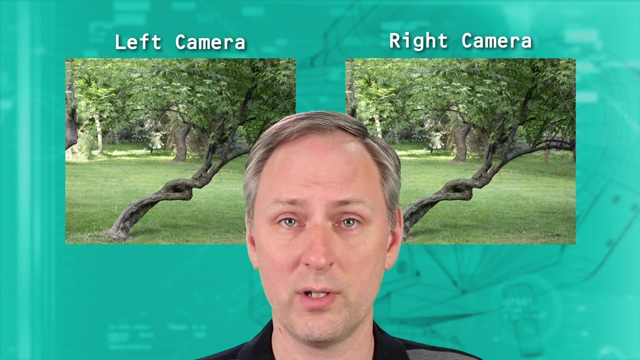 The next step is the image processing. This step takes a raw image and finds interesting parts. We can find edges or corners of objects, for example. For our example of trying to avoid hitting the tree, we need to find the tree in both images. 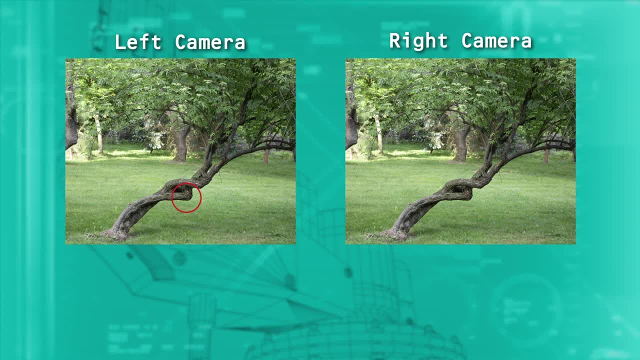 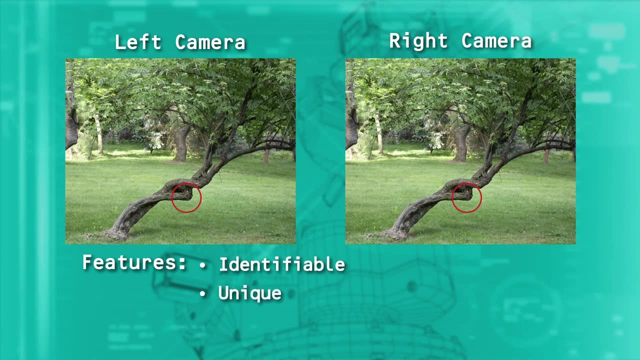 To do this, we look in both images for some common features of a tree. Features can be anything that the camera system can easily identify, such as unique patterns or corners. The key idea is that both cameras need to be aligned, So let's do that. 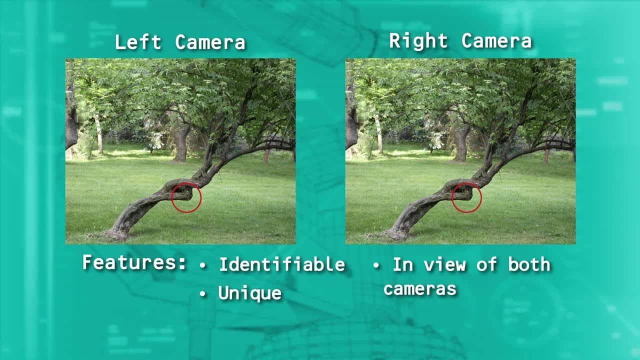 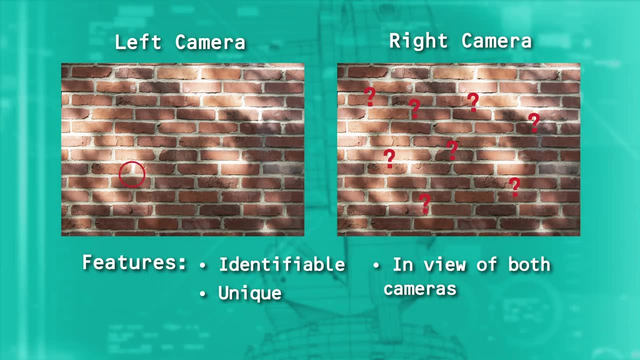 First, we need to be able to see and identify the features, and they need to be unique. The intersection point of some bricks and a brick wall might be easy to find, but it isn't unique, so you can't tell which junction you are looking at. 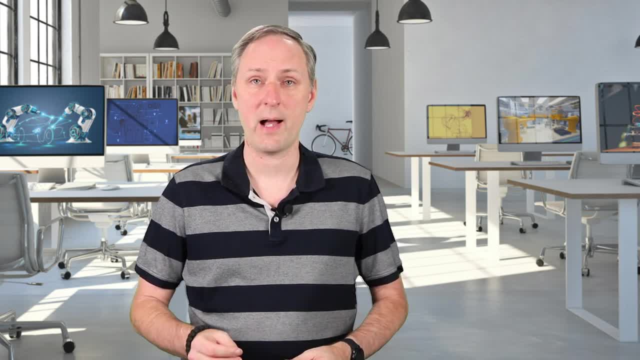 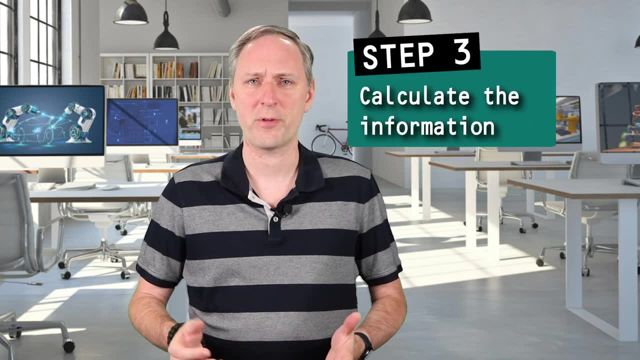 The final step is to analyze the images, That is, to calculate information from the features we've identified during the processing stage. One bit of information that the robot often wants to know is how far away are the things I can see from me. 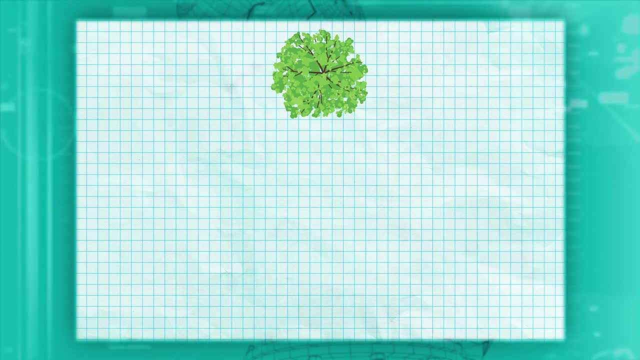 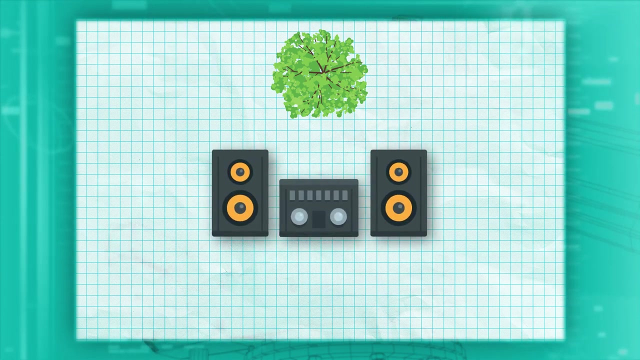 For our tree avoidance example. we want to be able to use these features to determine how far away the tree is so we can turn early enough to avoid a collision. One way of doing this is by using a stereo camera setup. Just like stereo sound produces different sound signals for your right and left ears. 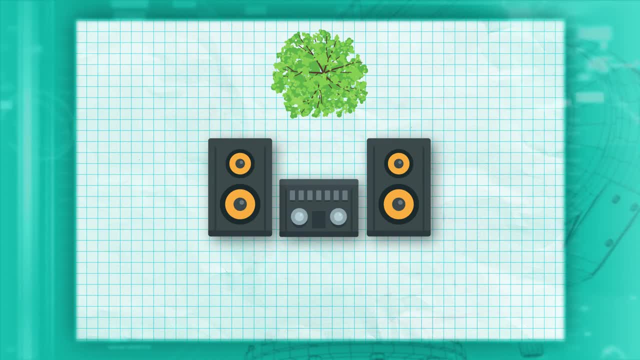 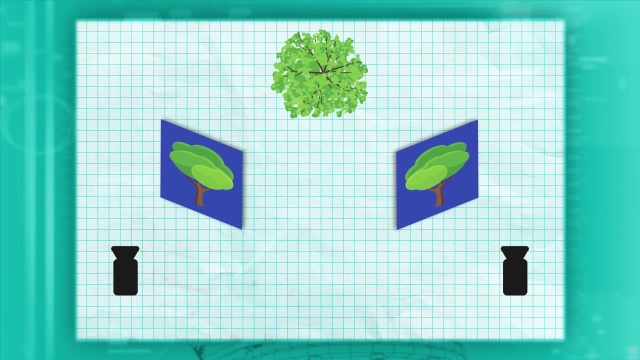 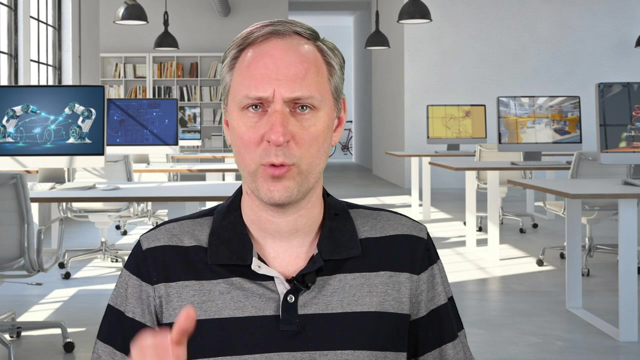 stereo cameras collect two simultaneous images with a right and left camera. The stereo cameras are used by the robot, are arranged parallel to each other and are a known distance. apart from the simultaneous images they collect, we can calculate where the tree is relative to the cameras. let's start by looking at our setup from overhead. we have our tree. 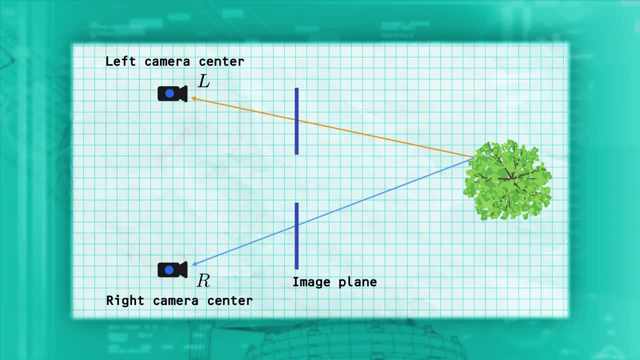 in front of the robot and two cameras on the robot mounted 50 centimeters apart. if there is a feature on the tree at a point P, then will appear on the image plane on the left camera, at point a, that point B for the right camera. we also 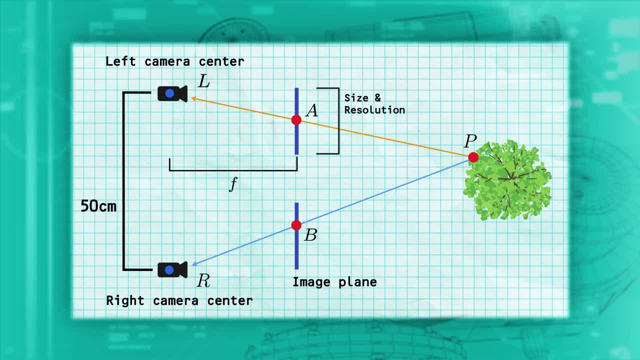 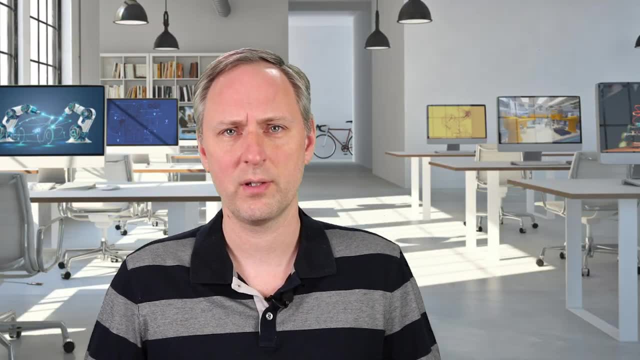 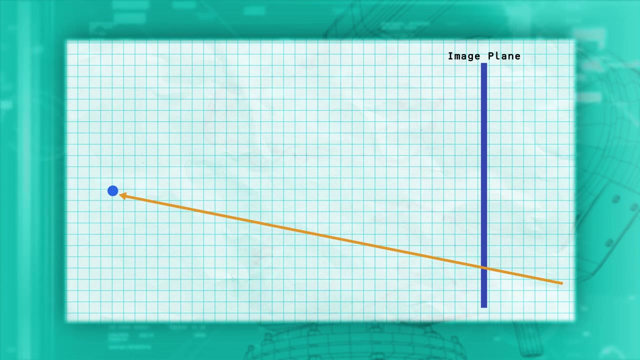 know the camera characteristics- focal length, sensor size and sensor resolution. so how can we determine the distance to the tree from this information? let's start by looking at the left camera up close. what we want to know is which way the orange ray is pointing. you want the equation for that line. let's set the. 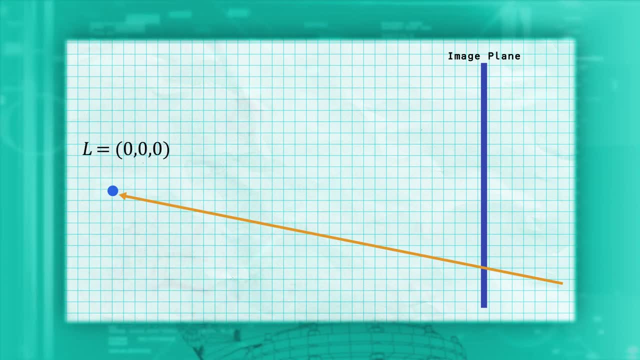 left camera center to be at zero point A and the left camera center to be at zero point B, and this is H, zero, zero, zero. we know the camera characteristics. in this case, the focal length is 50 millimeters, the sensor is 10 millimeters wide. there's 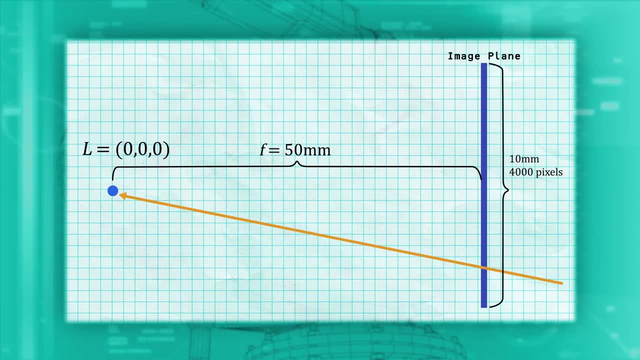 also 4 000 pixels wide. we know that the image plane is the XY plane, so the Z axis is perpendicular to that and points out in the same direction the camera is pointing. we also know where our point P shows up in our image. that is, we know. 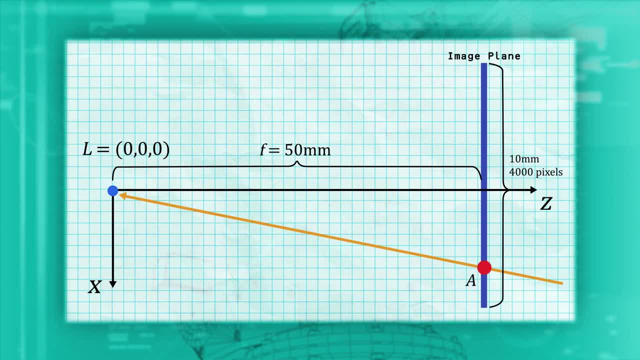 the x-coordinate for point A on the image plane. we know that the Z axis is goes through the middle of the image plane at point C, so the x-coordinate of C is zero. We also know that since C is in the middle of the sensor, it is 2000 pixels from the right. 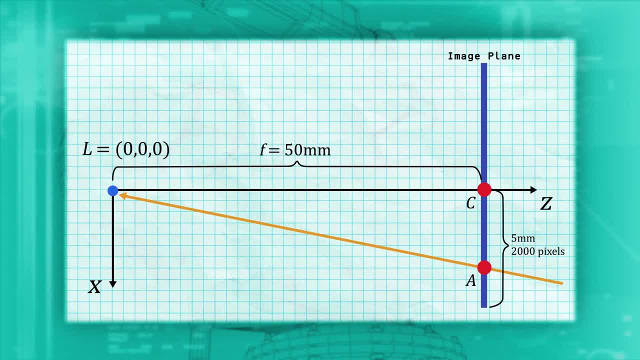 and left edge of the sensor. Let's say the feature we are looking at is at a pixel 2800, meaning it is 800 pixels to the right of center. Since the sensor is 10 millimeters wide, it is 5 millimeters from the center to the edge and also 2000 pixels from the center to the edge. 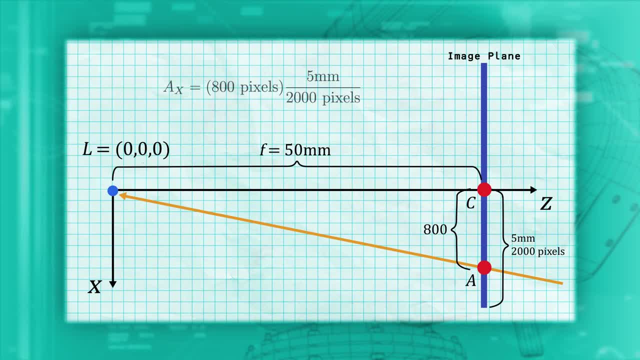 Taking our pixel coordinate for point A, we multiply by our ratio of 5 millimeters per 2000 pixels and get an x position of 2 millimeters. Now we know the location of the point on the image plane corresponding with our feature. x equals 2 millimeters and z equals 50 millimeters. 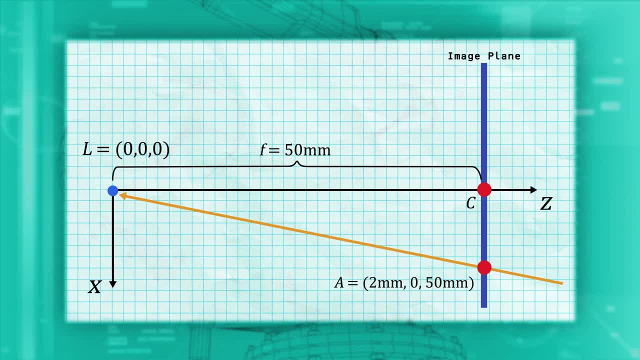 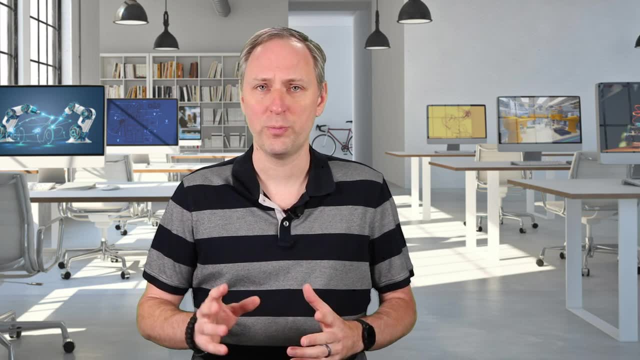 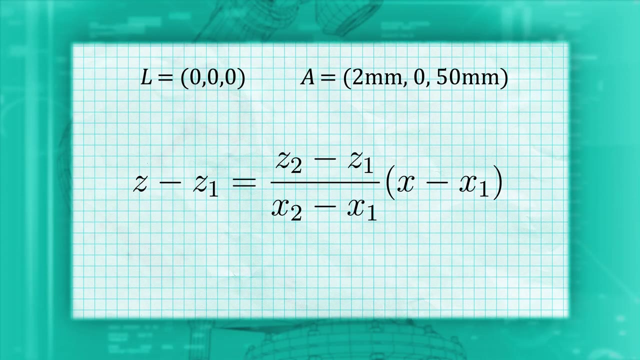 We also know that the line must go through the camera center. x equals 0.. From this we can create the equation for a line through two points: z minus z1 equals z2 minus z1 divided by x2 minus x1, multiplied by x minus x1.. 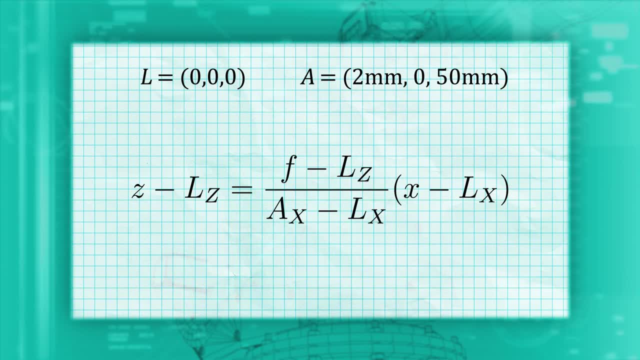 We already know some elements of this equation. We will set point 2 to be the feature on the image plane at point A, which is located at the focal length along the z-axis and at the x-coordinate we already found. We also know that the point 1 is the left camera center and is at 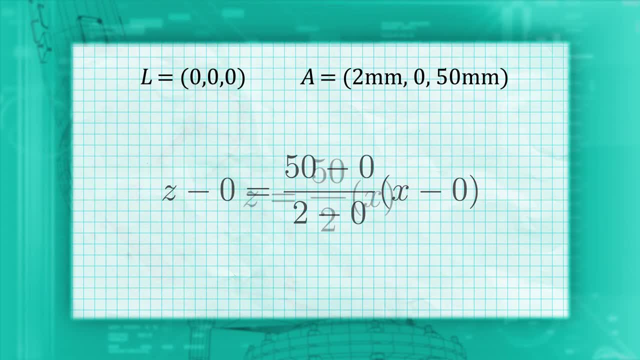 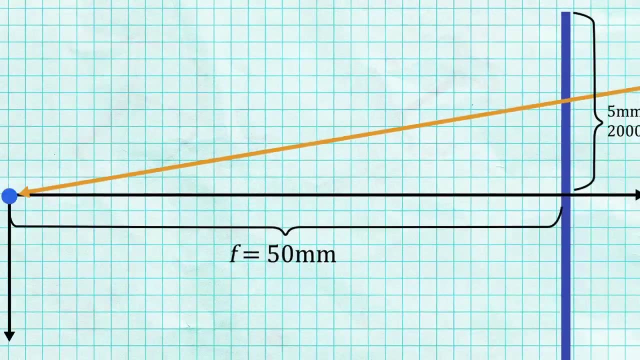 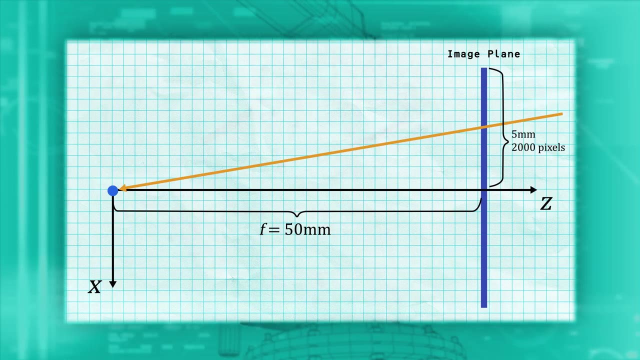 0,0.. We can simplify and substituting in our values, we see that we get: z equals 25x. We can do the same thing for the right camera. In this case, the camera center isn't at 0,0,0 anymore, since the camera is mounted in a different position. 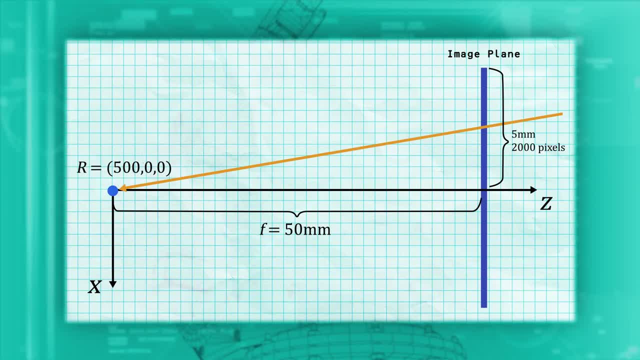 For our example, the cameras are mounted 50 centimeters apart, So the camera's center is at x equals 500 millimeters and z equals zero. Just as for the left camera, we will start with finding the distance from the sensor center to the point B. In this case, the feature is centered at an x coordinate of 800 pixels. 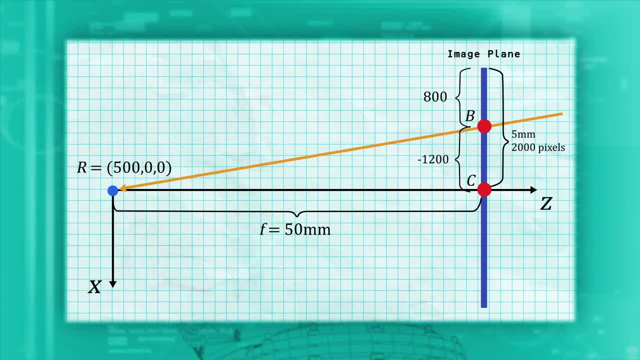 or 1200 pixels to the left of center, Multiplying negative 1200 by our ratio of 5 millimeters per 2000 pixels, we get an x position of negative 3 millimeters. However, remember that the origin is centered at the left camera center. so the true x position. 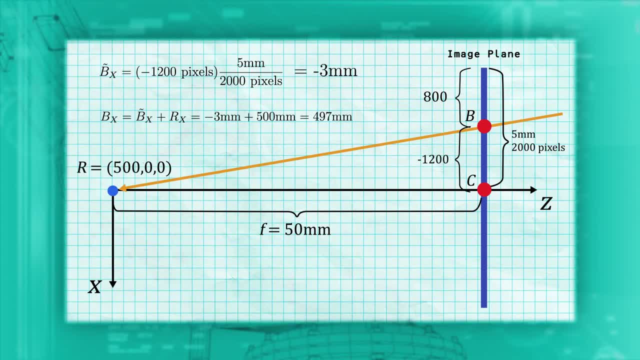 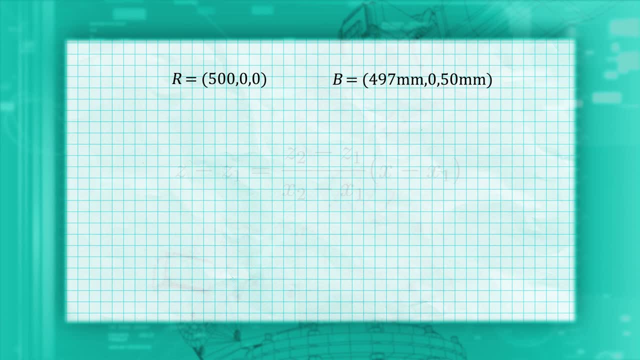 is 500 millimeters to the right or at 497 millimeters. Now we have our two points and can find our ray through point B. Starting with our equation for a line through two points, we know that the second point is the B coordinate and has a z value equal to the focal length. 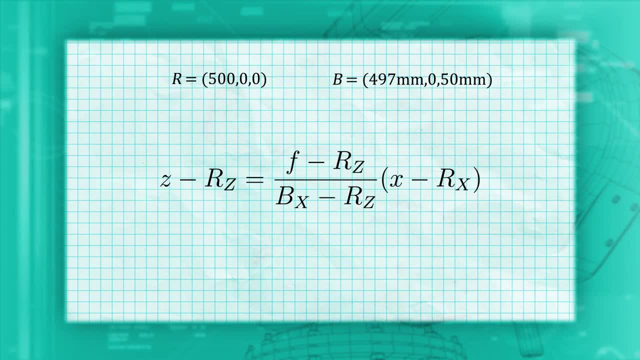 and point one is at 500, zero. We substitute in the values and simplify and we get our final equation: Z equals 8333 and one third millimeters minus 16 and two thirds times x. Now we have two equations with two unknowns. Z equals 8333 and one third millimeters minus 16 and two thirds times x. Now we have two equations with two unknowns: Z equals 8333 and one third millimeters minus 16 and two thirds times x. Now we have two equations with two unknowns. 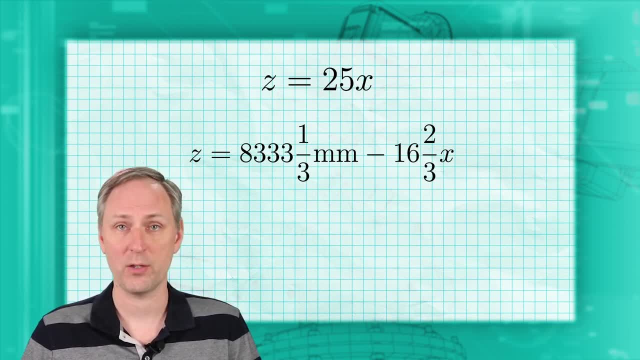 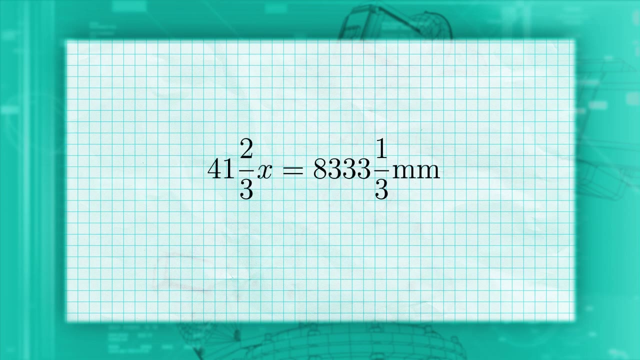 X and z the actual position of our point P in the real world. We can solve this system of equations by substitution, since they have z terms with a coefficient of 1.. We can then rearrange the equation to solve for x and we get a value of 200 millimeters. 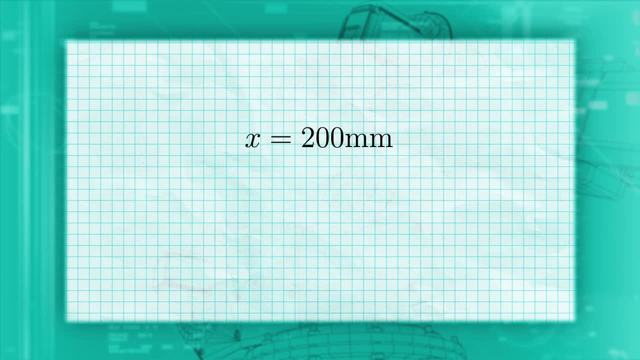 for x. Now substitute that back into either equation to find the z value. In this case we'll use the equation for the left camera And we find that the z coordinate is 5000 millimeters or 5 meters, which is about: 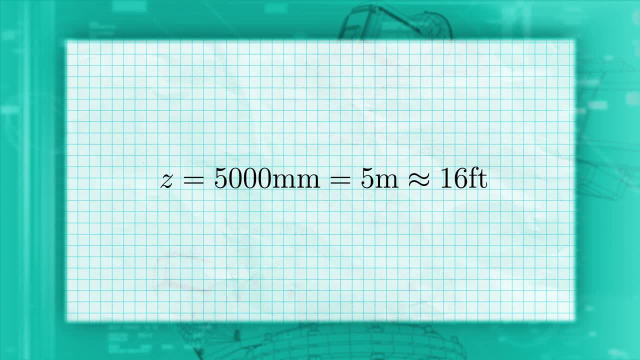 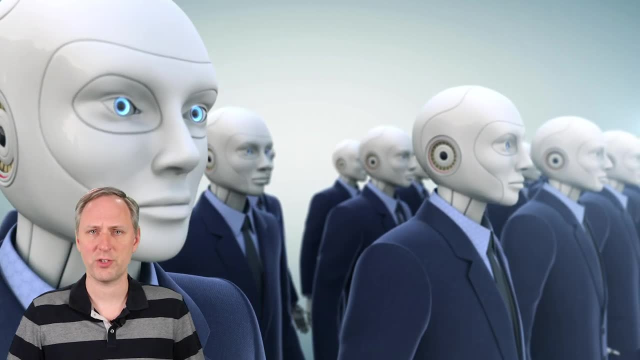 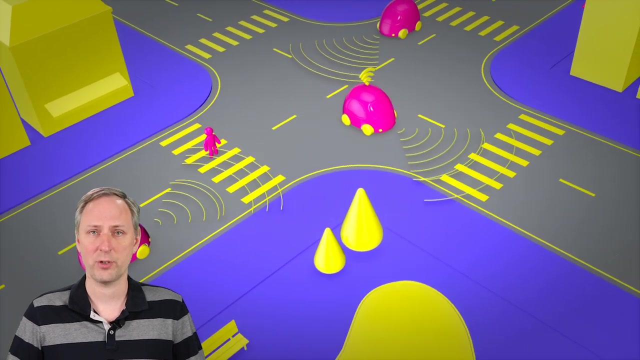 16 feet, And that is our answer. The tree is at 5 meters in front of our robot. With these skills, the robot can now put its vision system to good use: identifying the objects around it, interpreting signs in the environment and avoiding obstacles, all with